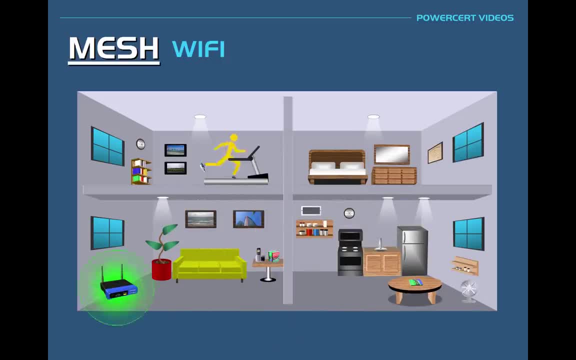 gives us the ability and freedom to do just that from all of our devices. However, sometimes the Wi-Fi signal can be a little spotty. For example, there might be areas in your home where the Wi-Fi signal is weak or it may be totally dead. Therefore, you're going to have slow internet speeds or you 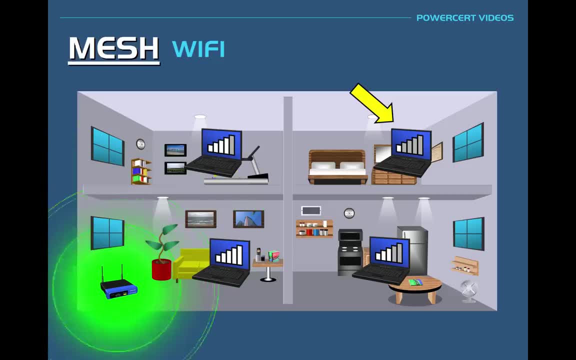 may not even have internet access at all, And this creates a lot of frustration. Now, this could be caused for several reasons. For example, it could be the construction of the building that's interfering with the signal, Or it could be the placement of the Wi-Fi router in the home. 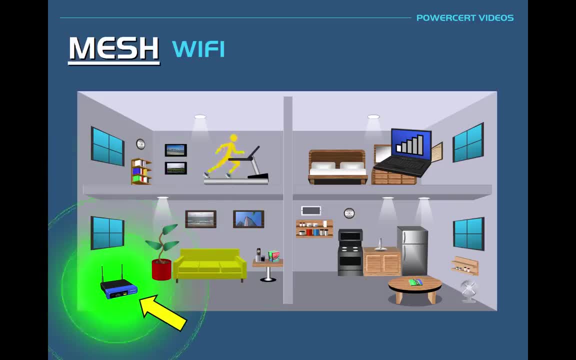 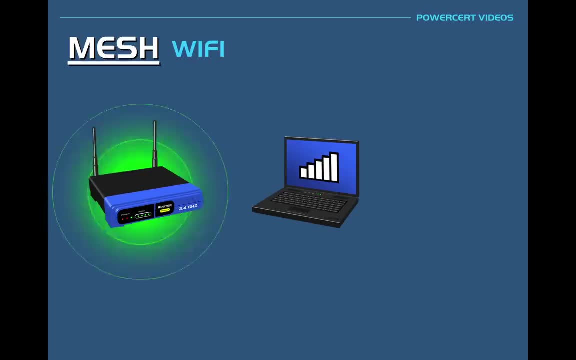 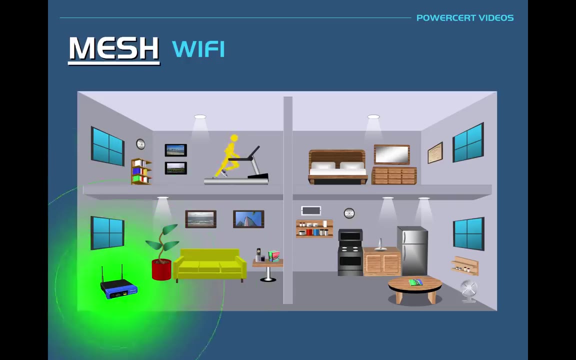 For example, if the Wi-Fi router is down here in the living room, you might have a weak signal or no signal up here in the bedroom, Because the further you get from the Wi-Fi router, the weaker this signal will be. So to remedy this problem, a lot of times people would buy a Wi-Fi extender to extend. 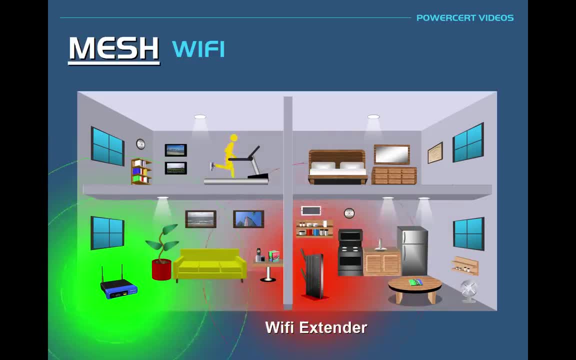 the Wi-Fi signal. Now, even though Wi-Fi extenders do work, the problem is is that Wi-Fi extenders create their own Wi-Fi network With their own separate SSID, So you would have to connect to the Wi-Fi router or the Wi-Fi extenders. 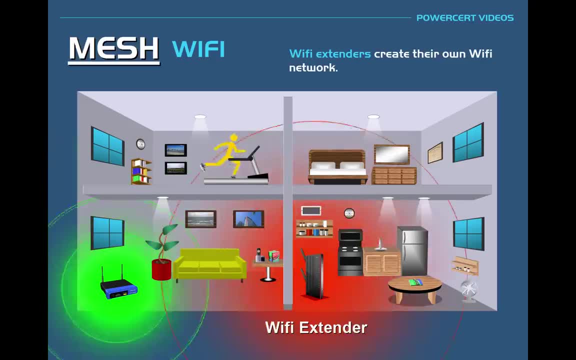 network depending on where you are in the home. So if you're closer to the router, then you would connect to the router, Or if you're closer to the extender, then you would connect to the extender. So this can be a little extra work. Or another solution could be is to place the Wi-Fi router to 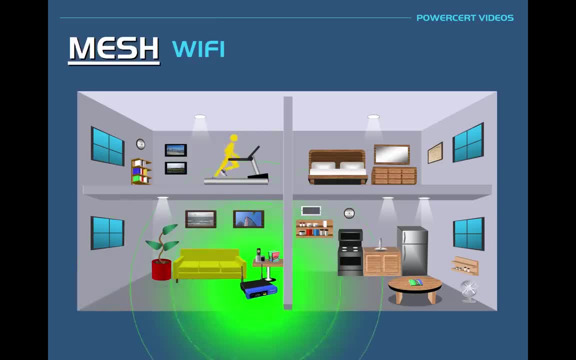 a different location in the home. an issue if the modem has to be in a certain place in your home because of cabling issues. But even if you were to place the wi-fi router to a better spot, the signal still may not be strong enough to cover the entire home. But there is a better solution for this, and this is by using 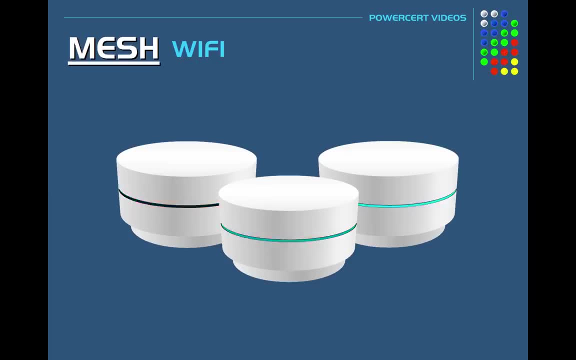 a mesh wi-fi system. Mesh wi-fi is the latest technology to solve the issue of weak or dead spot issues with wi-fi. A mesh wi-fi system is a group of routers or wi-fi points that are placed in different locations inside a home And it provides a blanket of wi-fi coverage all throughout.